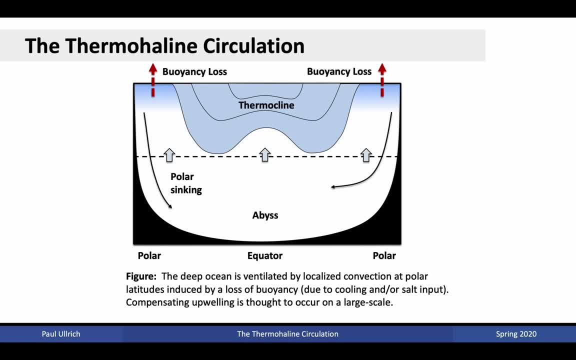 more homogeneous density profile and hence a propensity in the subpolar regions for deep convective events to occur. This deep convection is compensated for by a slow rising motion or upwelling that occurs through the extent of the oceans. An idealized depiction of the circulation. 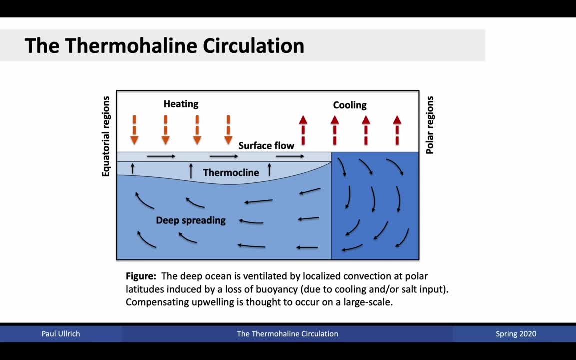 that arises is shown here. On the left-hand side, we have the equatorial regions. On the right-hand side, we have the polar regions. Heating from solar insulation occurs primarily in the equatorial and subtropical regions, whereas cooling occurs in the subpolar and polar regions. This means that we have a surplus of 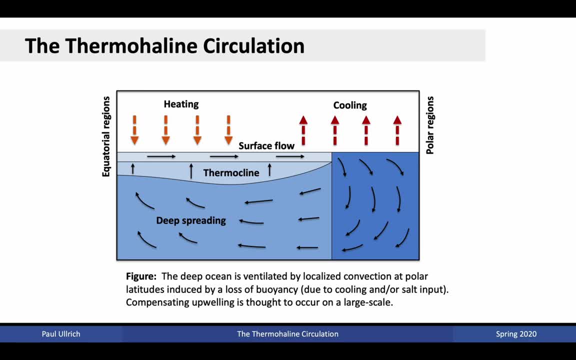 energy in the subtropics and a deficit of energy in the polar regions. In order to compensate for this, we must have a surface flow that is then responsible for transporting warm ocean waters from the equatorial regions towards the polar regions. Because of buoyancy loss in the polar 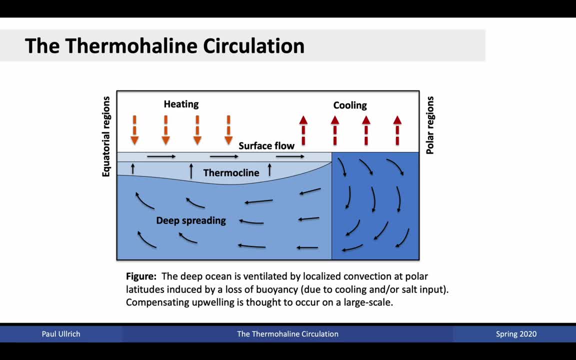 regions. we must then have sinking waves ocean. that occurs here. This then drives a deep underlying oceanic currents. These oceanic currents then recirculate back towards the equatorial regions, where large-scale upwelling is then responsible for completing the circuit and bringing that water back to the surface. 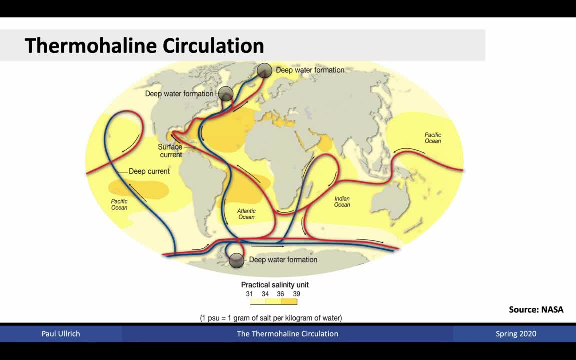 Because of the buoyancy loss that occurs in these subpolar regions, we end up driving large-scale oceanic currents that have global extent. Here we see a depiction of those currents, with red lines showing surface currents or surface transport of warm water through the ocean basins and the blue. 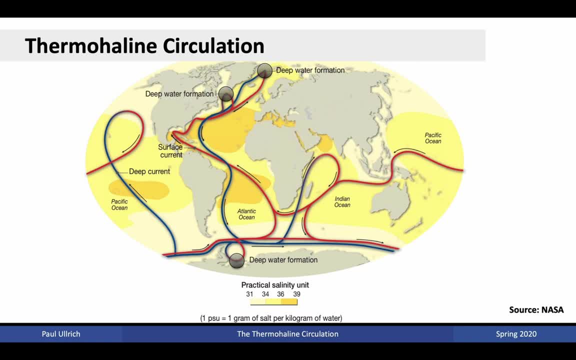 lines showing deep water and deep water transport. We see that only in three regions we have deep water formation. that is where these warm surface currents sink to depth in order to push the deep ocean currents Throughout the ocean. however, we do have upwelling where these deep ocean 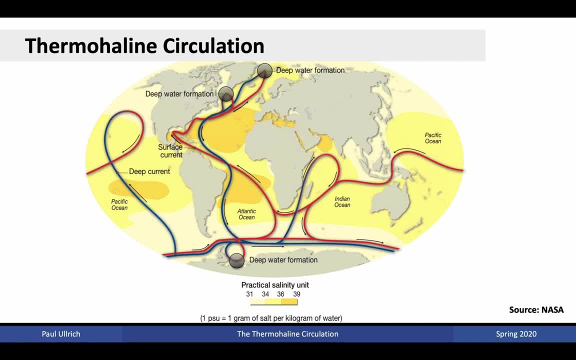 currents sink to depth in order to push the deep ocean. currents are returning to the surface, although this primarily occurs in the subtropics and equatorial regions, Since the oceans are bounded on each side of the basin, of course, this is very different. 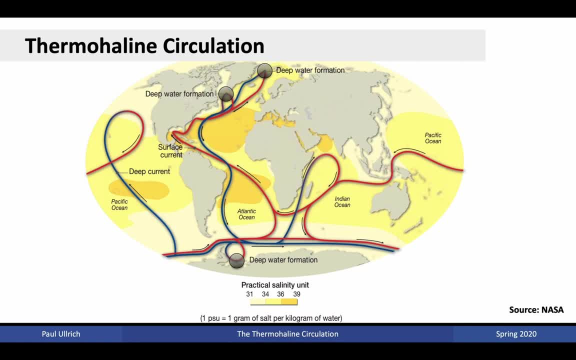 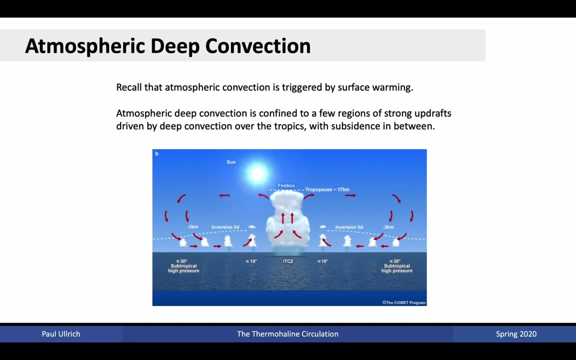 than the types of exchanges that we see in the atmosphere. That is, the oceanic movements are constrained by those continental boundaries, hence giving rise to this entangled pattern of oceanic currents. Recall that in the atmosphere, convection is primarily triggered by surface. 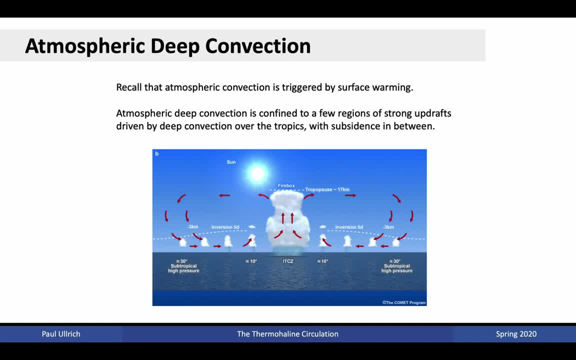 warming In the oceans. it's the opposite, In fact. we need to have surface cooling in order to trigger convection, because the energy exchange occurs at the top of the ocean rather than at the bottom, as it does in the atmosphere. Atmospheric deep convection is confined to a few regions of strong 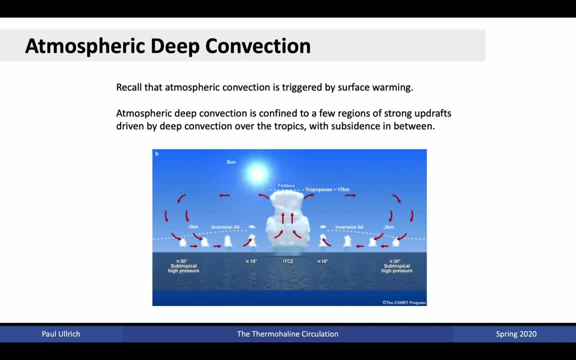 updrafts driven by deep convection over the tropics, with regions of subsidence in between The oceans, on the other hand, will be stabilized by the presence of surface warming, and so it's essentially impossible for deep convection to occur in the atmosphere. So in the oceans we have 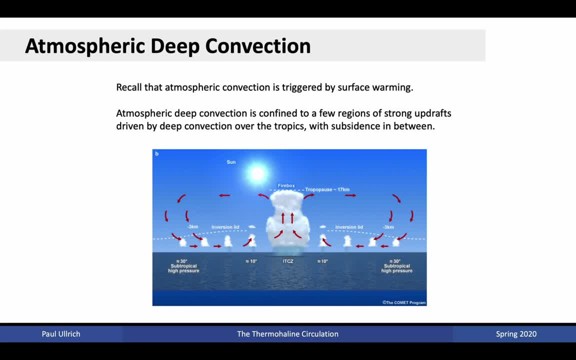 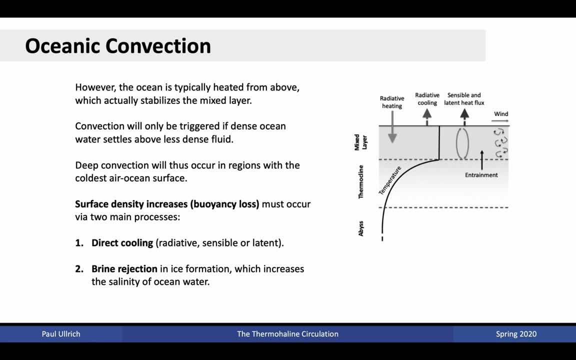 deep convection to occur in the equatorial regions of the ocean. Since energy exchange occurs at the atmosphere-ocean boundary, warming from above because of solar insulation will cause stabilization of the mixed layer, consequently preventing deep convection from occurring. Convection will only 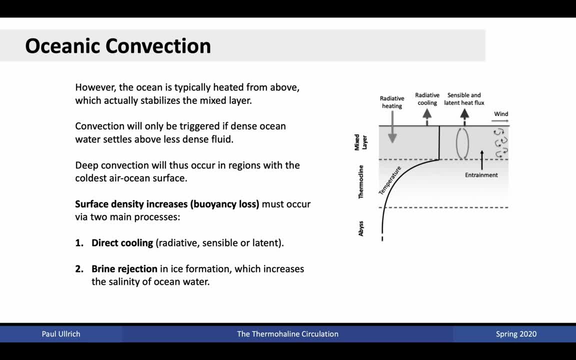 be triggered in the ocean under very limited conditions in which the water above ends up being more dense than the underlying waters. Deep convection thus requires a big amount of of factors that all contribute to increasing density in the surface layer. Deep convection must 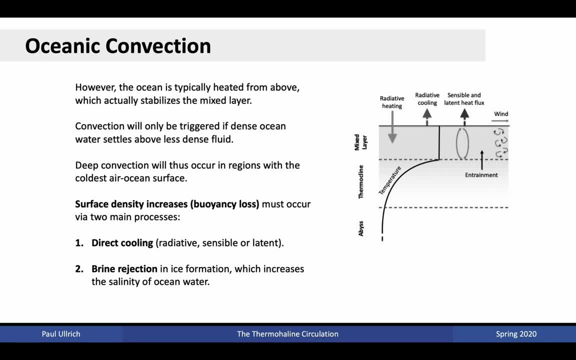 thus occur in regions where we have the coldest air-ocean surface. There are other processes that then drive this density increase, including direct cooling in the form of radiative sensible or latent heat exchange, as well as brine rejection, in which the formation of sea ice 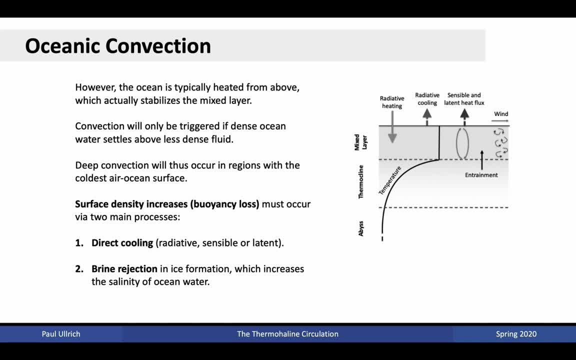 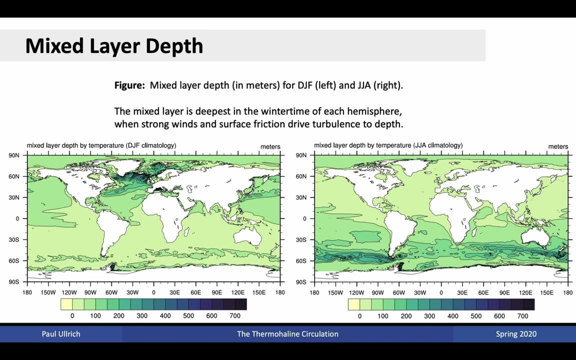 rejects salt, consequently leading to an increase in the salinity of the ocean. The mixed ocean depth also gives some perspective on where these regions of deep convection are likely to occur. During the winter season of each hemisphere, we get the deepest mixed layer. 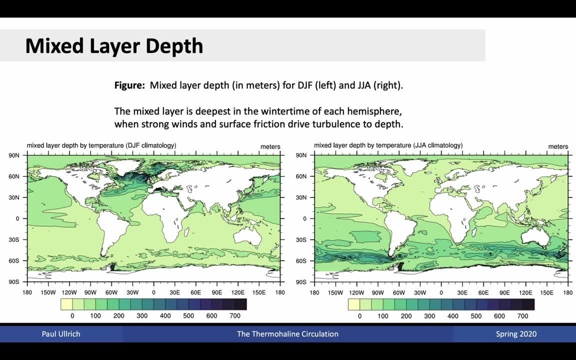 depths occurring at these subpolar latitudes. These are regions in which the mixed layer has the greatest homogeneity to depth. In these regions with greatest homogeneity, we then have the potential for deep convection events to occur. Notice in the diagram on the left-hand side that the deepest mixed layer depths occur in the. 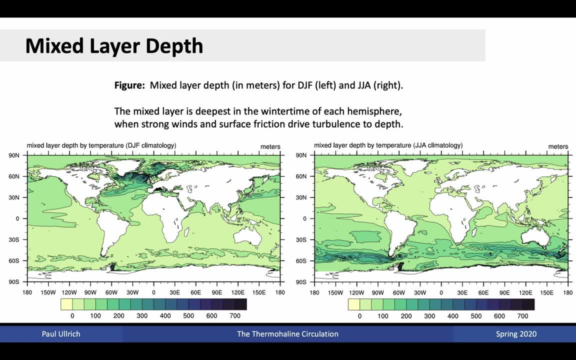 North Atlantic during the Northern Hemisphere winter season, whereas during the Northern Hemisphere summer season the deepest mixed layer depths occur in the Wendell Sea at the southern extent of the Atlantic Ocean, But we also have significant mixing that occurs along the extent of the Antarctic circumpolar current, The three primary regions for deep oceanic convection. thus, 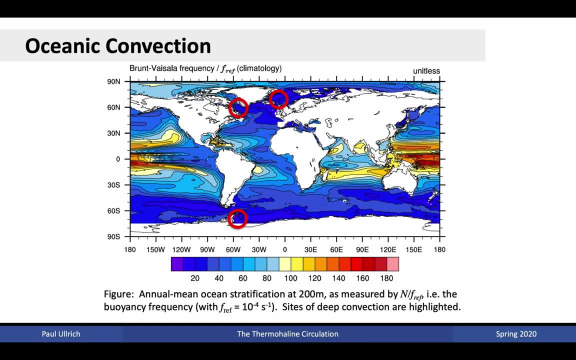 occur in the North Atlantic during the Antarctic circumpolar current, In the Northern Hemisphere, in the Labrador Sea, in the North Atlantic to the northeast of Iceland and in the Wendell Sea in the South Atlantic. Annual mean ocean stratification here is shown. 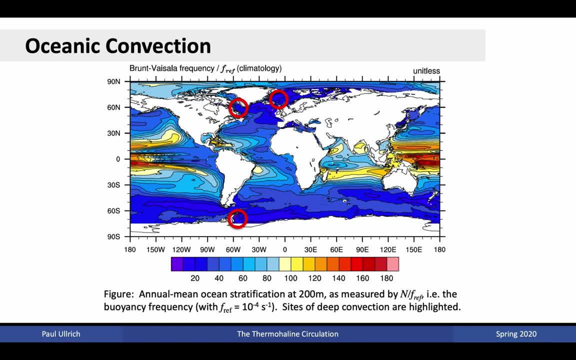 at 200 meters. In the regions with the darkest blue and nearly purple colors, we have the lowest Brunt-Visala frequency. These low Brunt-Visala frequencies are associated with near homogeneity of the density through these regions In order to have deep convection. events occur in the 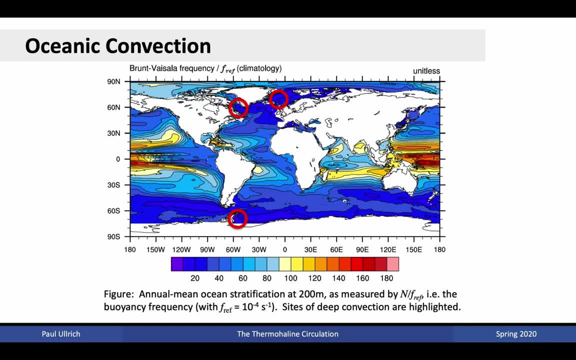 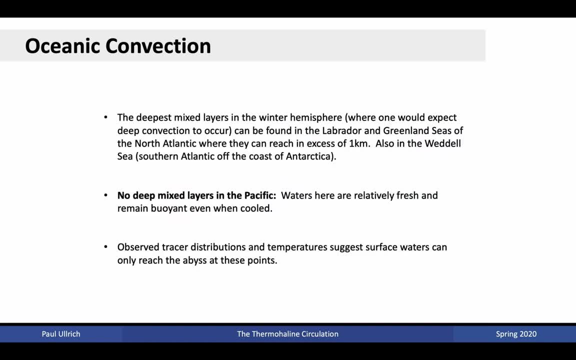 North Atlantic we must have that the Brunt-Visala frequency is approximately less than about 20 in these normalized units. So, to summarize, the regions of the world with the deepest mixed layers can be found in the Labrador and Greenland Seas of the North Atlantic, where these mixed 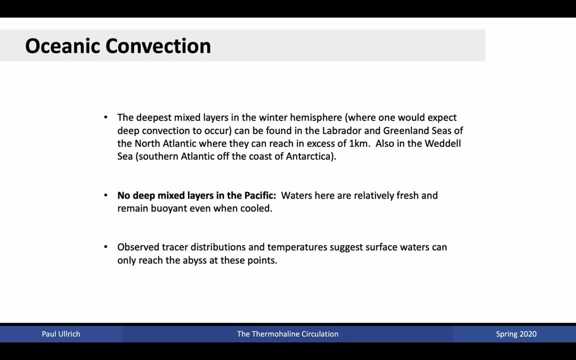 layer depths can reach in excess of one kilometer. Also, we can see these deep mixed layers in the Wendell Sea, along the southern Atlantic, off the coast of Antarctica Notably, there are no deep mixed layers that occur within the Pacific. In the Pacific, the waters are relatively fresh compared. 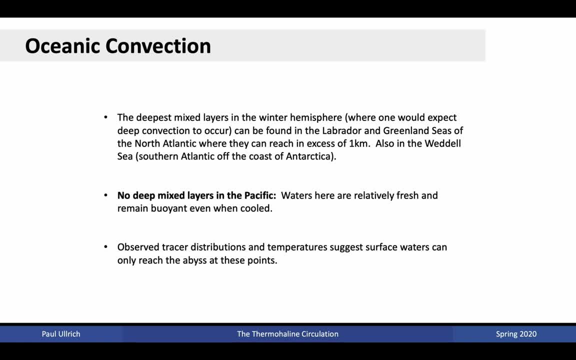 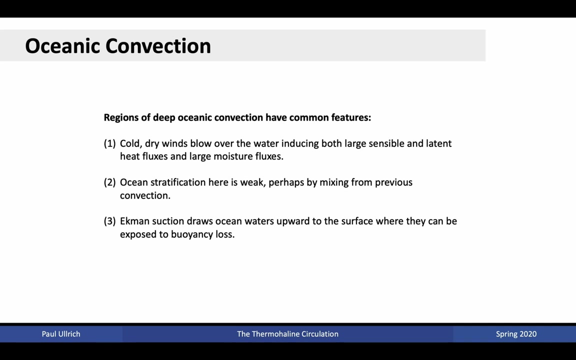 to the Atlantic and consequently remain buoyant even when cooled. Consequently, there's very little deep convection that occurs within the Pacific Observed tracer distributions and temperatures suggest that surface waters can only reach the abyss in these three locations identified. These regions of deep oceanic convection all have several common features associated. 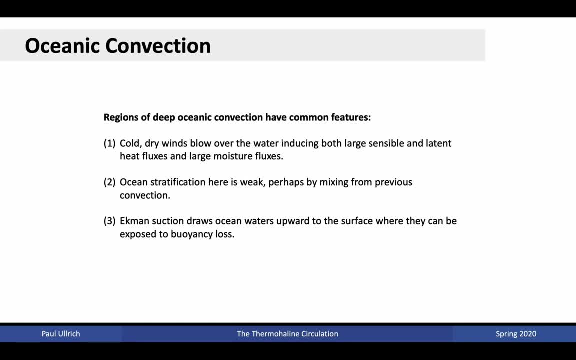 with them. We must have cold, dry winds that blow over the water, inducing large, sensible and latent heat fluxes as well as large moisture fluxes. that is, evaporation from the ocean surface. Recall that evaporation from the ocean surface rejects the coldest molecules of water. 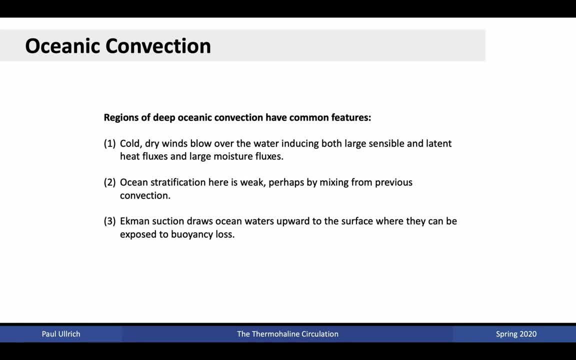 Consequently, by withdrawing the more energetic molecules, we end up cooling that surface. Secondly, the ocean stratification in these regions is weak, which likely occurs because of mixing from previous convective episodes, That is, through turbulent mixing through the top layers of the ocean. here we effectively set up a homogeneous density profile that 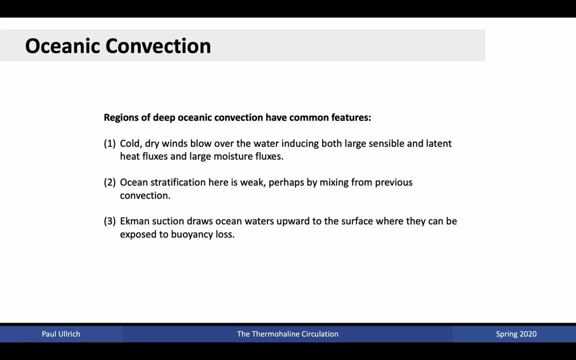 provides an initial state for deep convection to occur. Finally, we have Ekman suction that occurs in these regions. Recall that Ekman suction is common in the subpolar and polar latitudes. This is responsible for then drawing ocean waters upwards to the surface in order to 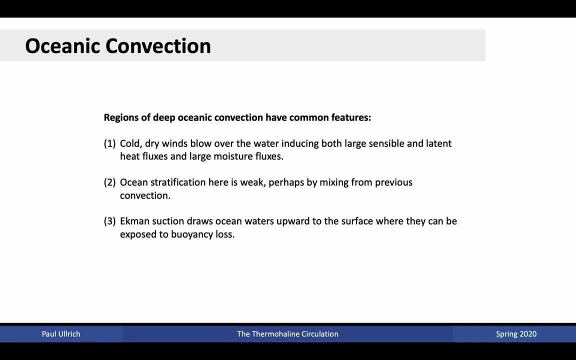 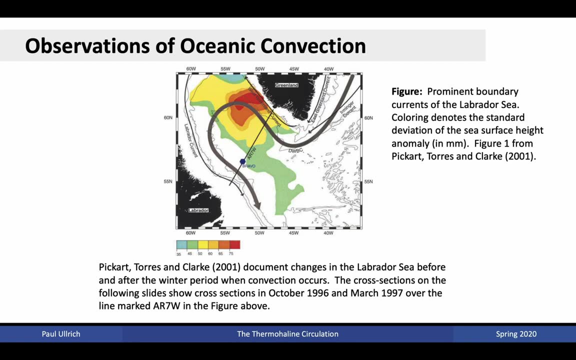 bring those cold ocean waters up to the surface. This is a very important feature of deep convection. where deep convection is observed in practice, However, one such season of deep convection was observed and documented by Pickard Torres and Clark in their 2001 paper. In the next two slides: 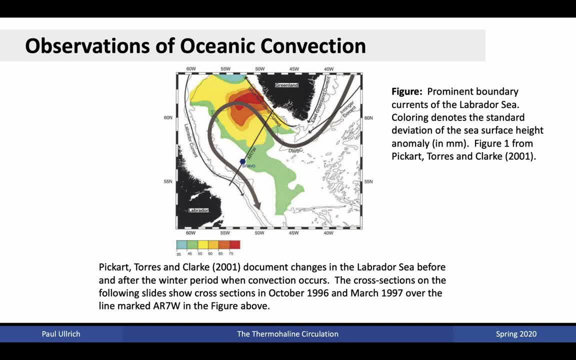 we're going to see cross-sections before and after deep convection, Before and after a northern hemisphere winter season, taken via a ship crossing a transect between Labrador and Greenland in the North Atlantic. The cross-sections were taken on October 1996 and March 1997 over this line, AR7W, shown here. 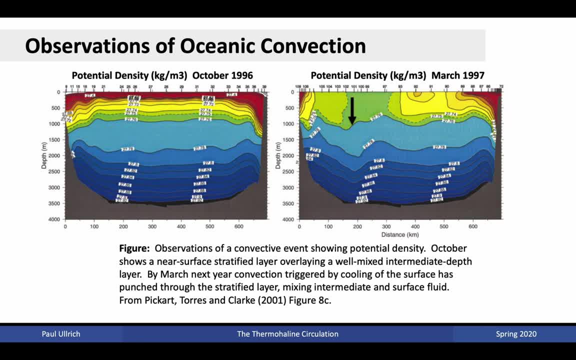 On the left hand side we see the potential density profile on October 1996.. On the right hand side we see the potential density profile on March 1997.. Less dense waters are shown in warmer colors and more dense waters are shown in cooler colors. 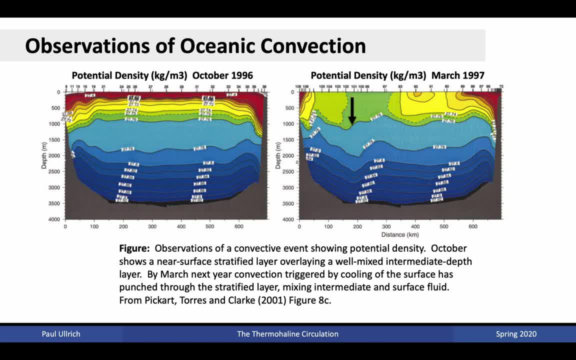 What we see is that over the course of this winter season, through a process of heat loss from the surface as well as brine rejection, we have an increase in the near surface density of the fluid. What likely occurred over the winter season is vertical mixing through deep. 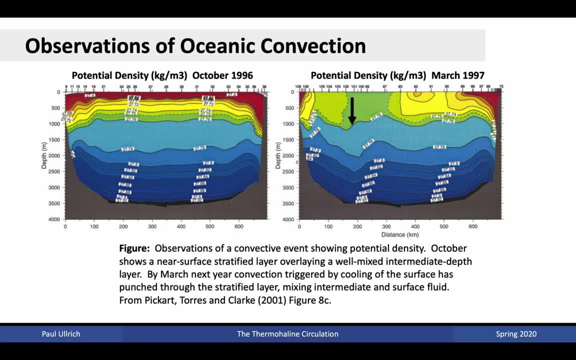 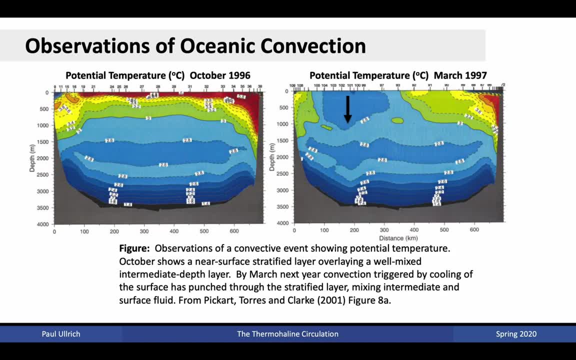 convection event that was then responsible for leading to homogenization through this column. The black arrow here indicates a position where that deep convection event occurred. Here we again see potential temperature for October 1996 and March 1997.. Again we see. 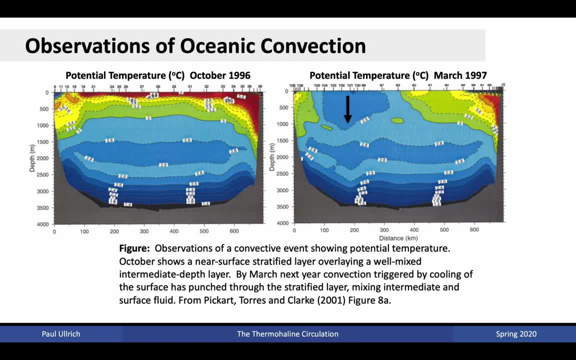 basically homogenization of the potential temperature through the region where deep convection is suspected to have occurred. Note that they did not observe the deep convection event directly, as that would be quite difficult and would require conditions where, essentially, ship travel would be impossible. Namely, these deep convection events occur during, incredibly, 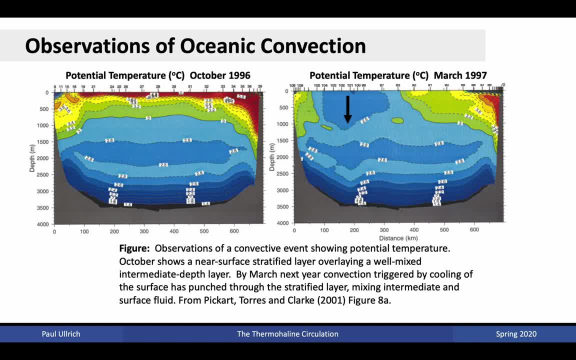 cold storms and under rough conditions, where traversing this particular region of the world is very difficult. Nonetheless, by observing conditions both before the winter season and after the winter season, we were able to see many of the fingerprints that would be indicative of deep convection events. The mixed layer depth that was then observed in 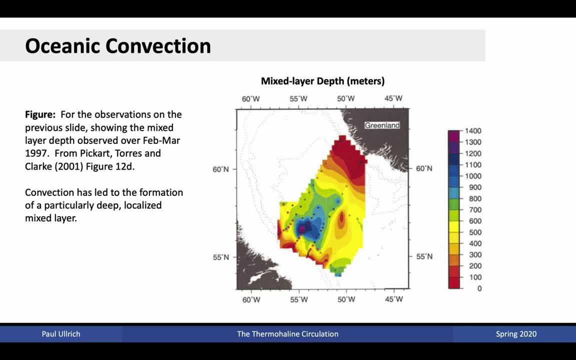 February to March 1997 indicated that we basically had deep homogenization through this region close to the Labrador coast. Where we see the purple here in this particular diagram is where it was expected that waters from the near surface were carried to very deep in the Atlantic Ocean. Convection hence has led to the formation here of a particularly 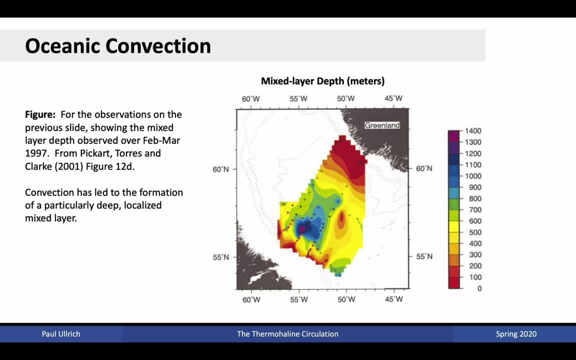 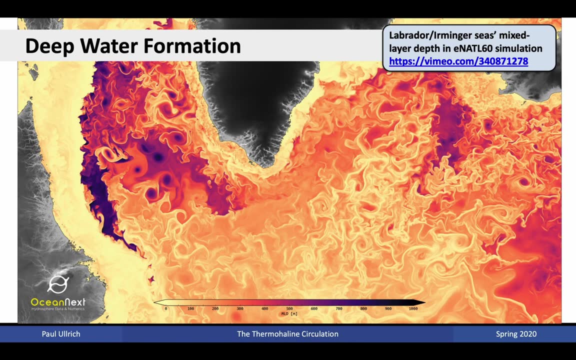 deep and localized mixed layer. This particular region is known for its propensity in order to form these deep mixed layers and, consequently, for driving an exchange of ocean waters from the surface to depth. Although we may not have observations, available computer simulations at very high resolution. 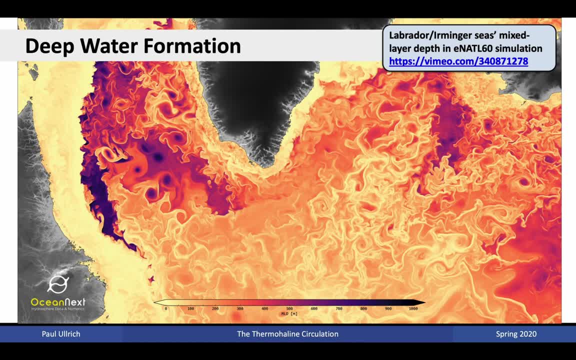 have backed up the theories behind deep water formation in this region. Here we see a snapshot from a simulation performed with the NEEMO model at depth in the North Atlantic. If you want to watch this video, follow the link above. This shows the mixed layer depth over: 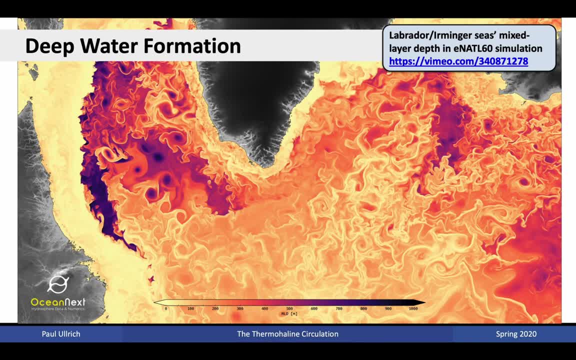 time over the course of a whole winter season. The regions of darkest color or the darkest shades of purple correspond to regions where we have deep water formation in the region. In the first phase we see deep layers of oceanic convection in the water. There is no apparent 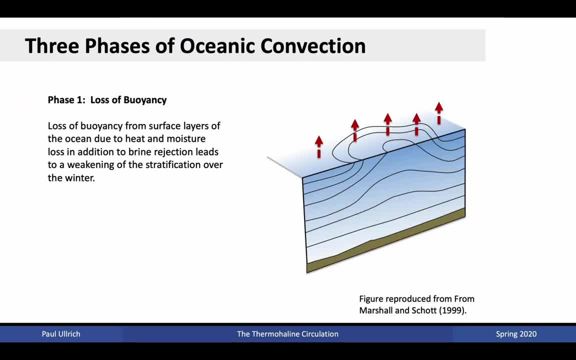 change in temperature during this phase due to the heat and moisture loss. From a theoretical perspective, there are essentially three phases that drive oceanic convection. Phase one: as we get into the early stages of the winter season, we have a loss of buoyancy. 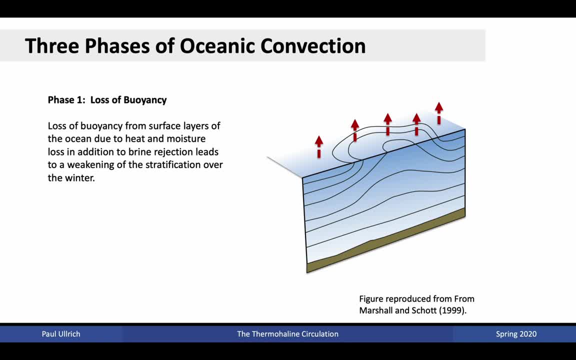 from the surface layers of the ocean due to heat and moisture loss. Namely, we have sensible latent and radiative heat loss that occurs from the near surface, leading to cooling. occurs under particularly strong winds, which drive mixing and evaporation from the oceanic surface. In addition, sea ice formation, driving brine rejection. then 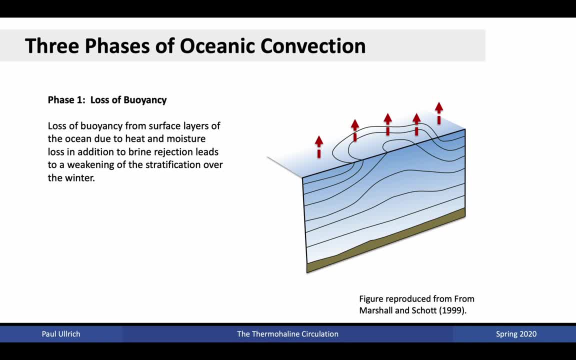 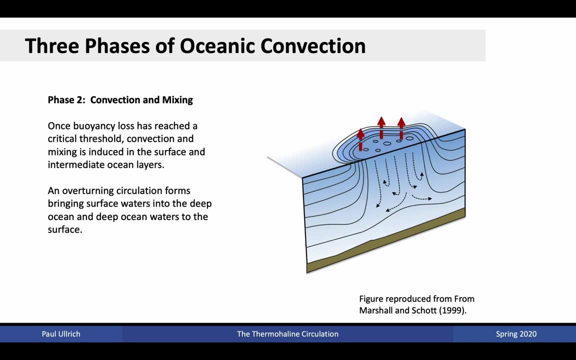 leads to increased salinity in this near-surface ocean layer, consequently driving up the density even further. This leads to a weakening of the stratification over the winter and hence sets up conditions for deep convection to occur. When conditions are just right, namely once we have a 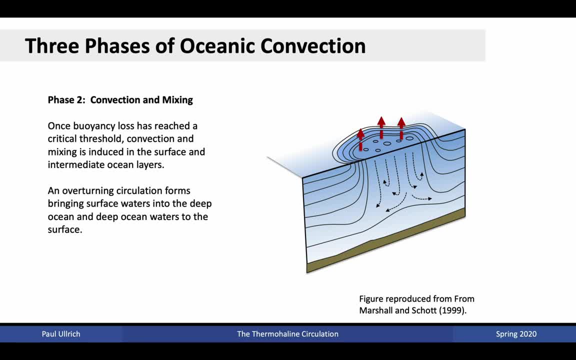 sufficiently deep mixed layer, as well as homogenization of the ocean, we can then trigger an oceanic deep convection event. Namely, once this buoyancy has reached a critical threshold, convection and mixing are induced in the surface and intermediate ocean layers. An overturning circulation forms because 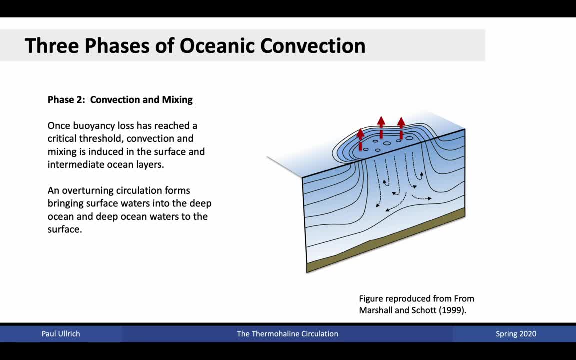 much like what we saw in the case of the atmosphere, a system such as an oceanic sea Editor, where there is low-density water left inside the ocean, we end up in an unstable arrangement which can trigger Rayleigh-Binnard type convection. In this particular arrangement we have 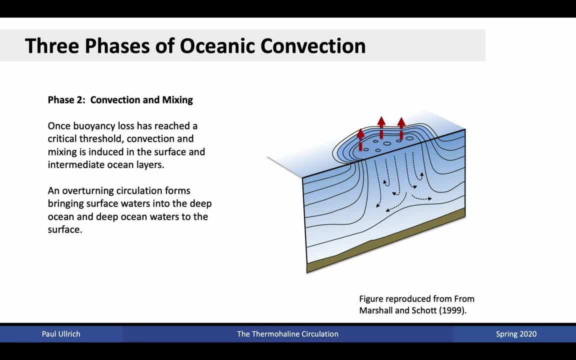 dense heavy ocean waters sitting on top of lighter ocean waters. The overturning circulation then brings surface waters to depth into the deep ocean, as well as bringing those deep ocean waters with lower density up to the surface. the deep ocean waters are now exposed to water that was recently in contact with the atmosphere. 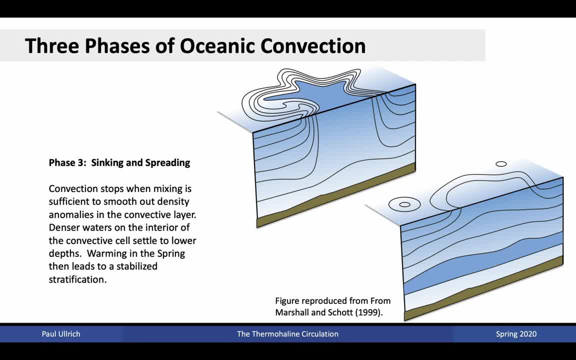 The convective event finally concludes when the mixing is sufficient in order to smooth out the density and bring the vertical profile back to neutrality. Once this occurs, the denser waters in the interior of the convective cell will then settle to lower depths, Warming in the spring. 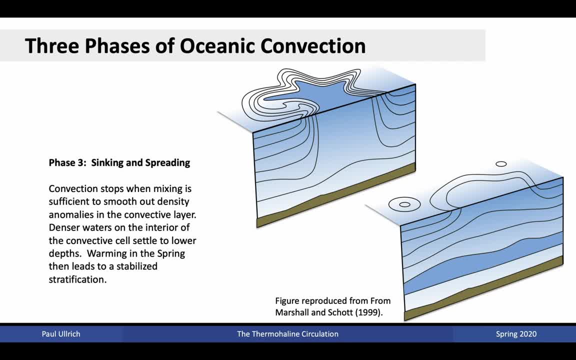 then leads to a stabilized stratification, namely once the winter conditions cease and we end up with increased solar insulation in this region of the world. we then end up with surface warming, which, as mentioned before, is then responsible for triggering stabilization through the oceanic column. Consequently, the ocean waters that were once at the surface earlier in the winter season. 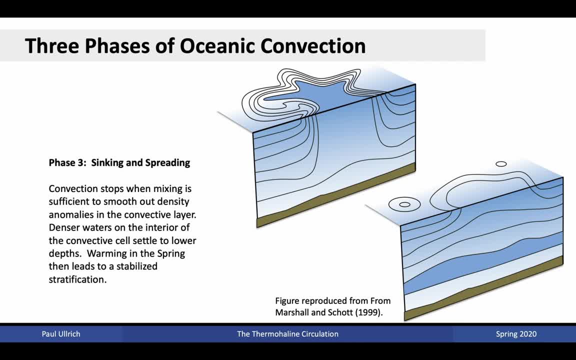 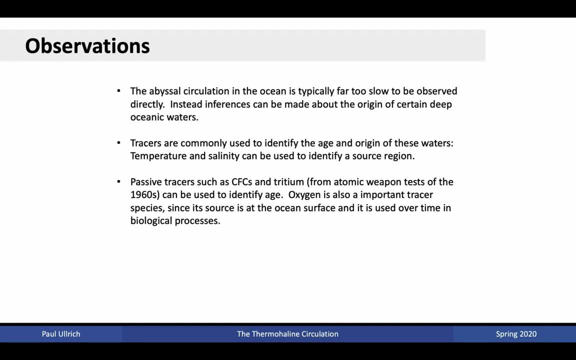 have now been brought to depth and thus can play a role in broader transport through the ocean deep currents. The ocean waters that have now reached depth will now circulate through deep ocean currents. However, it's very difficult in order to find direct evidence of this circulation, Namely the abyssal. circulation in the ocean is typically 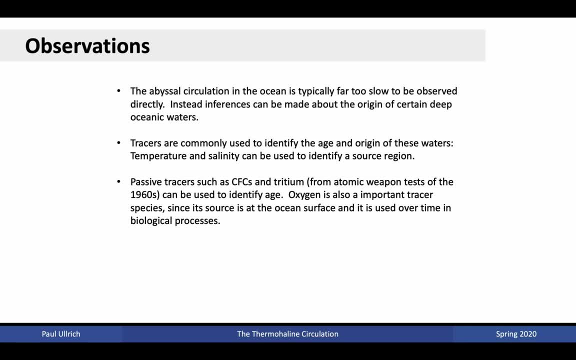 far too slow in order to be observed directly, with typical abyssal current speeds on the order of centimeters per second. Instead, inferences can be made about the quality of these circulations by looking at the origin of certain deep oceanic waters, That is, particular tracers can be used to. 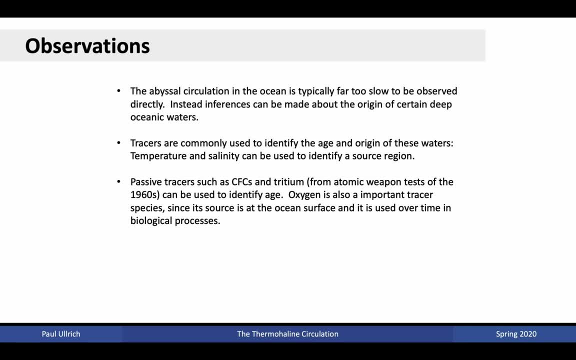 identify the source point of certain oceanic waters. We can look at temperature and salinity in order to identify a source region by comparing that to the source point of the ocean. Passive tracers such as chlorofluorocarbons and tritium from atomic weapon tests in the 1960s can 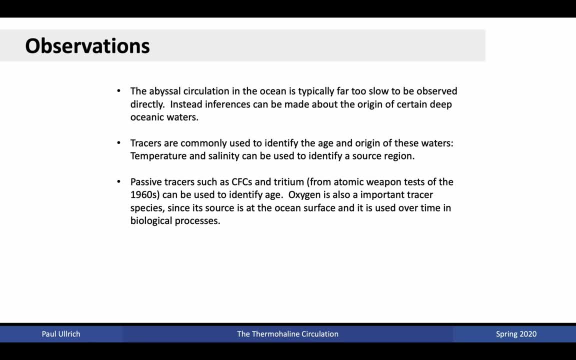 also be used to identify age. Here, age refers to the last time that those oceanic waters made contact with the surface. Thus, ocean waters that are one year old last made contact with the surface one year ago. Because the oceanic circulations are so slow, even injections of CFCs and 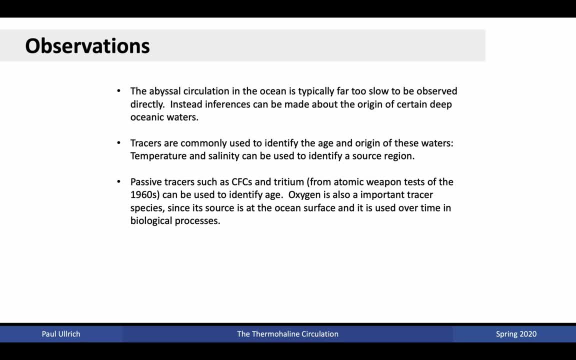 pir extracts from the 1960s have only partially transited through the Atlantic. Oxygen is also an important tracer species, since it's indicative of the last time that ocean waters made contact with the surface. Biology within the ocean slowly consumes the oxygen content of the water. Consequently, since it's used up over time, the less oxygen 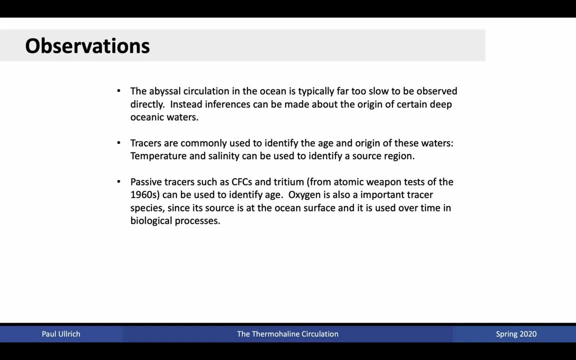 there is in the water, the likely older that water is. Let's look at each of these tracers. in order to examine the fingerprints of each of these tracers of the Atlantic, They look similarly similar to the tracer on the구요io slide. 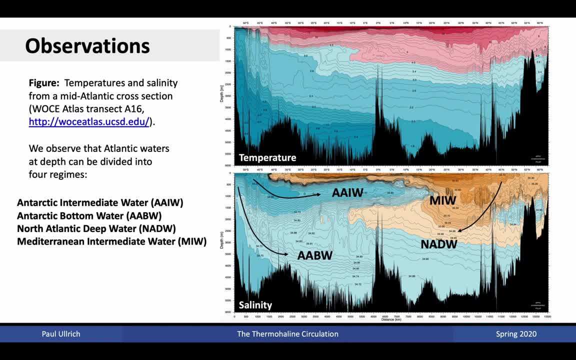 deep ocean circulation. On the top plot here we see the temperature profile of the Atlantic Ocean taken from the WOCE Atlas along transect A16.. For more plots like this you can check out the Atlas at the link provided here. The warmer ocean waters of the near surface are primarily driven. 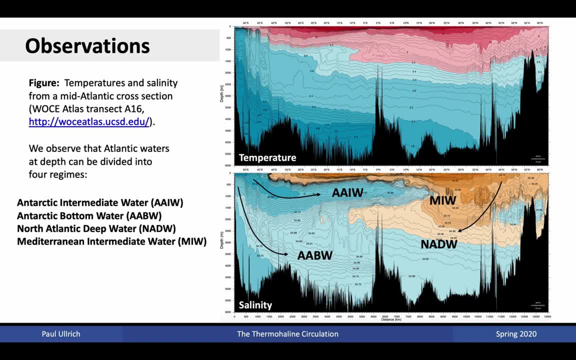 by Ekman: pumping and suction. It's primarily the deep waters where we're interested in performing our fingerprinting In particular, if we look at the salinity plot on the bottom, we can observe that the Atlantic waters at depth can be roughly divided into four regimes, based on their origin. 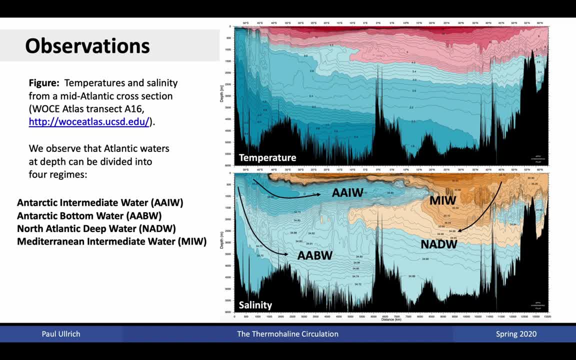 We have Antarctic Intermediate Water, typically denoted AAIW, Antarctic Bottom Water, denoted AABW, North Atlantic Deep Water, denoted NADW, and Mediterranean Intermediate Water, denoted MIW. In the salinity plot we see clear evidence of different circulations that are then responsible. 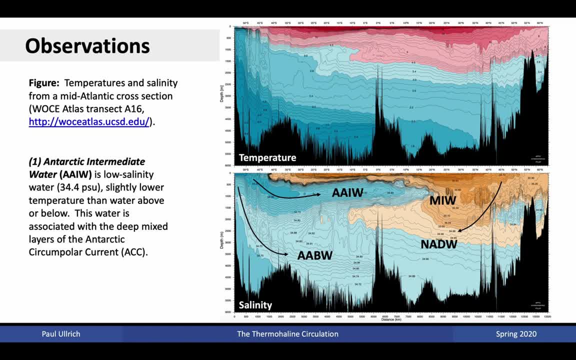 for driving differences in salinity at depth. The first type of water is the Antarctic Intermediate Water. This is relatively low salinity water, typical values of 34.4 practical salinity units and slightly lower temperature than the water above and below. This water emerges because of deep mixed layers that occur naturally in the 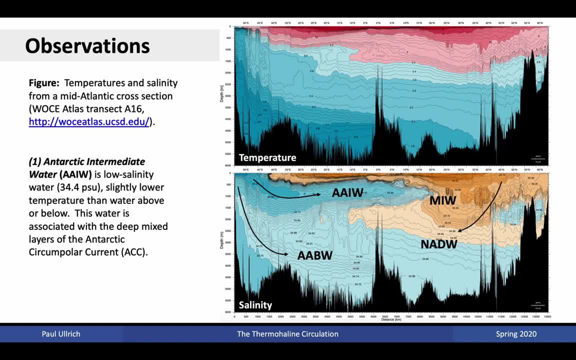 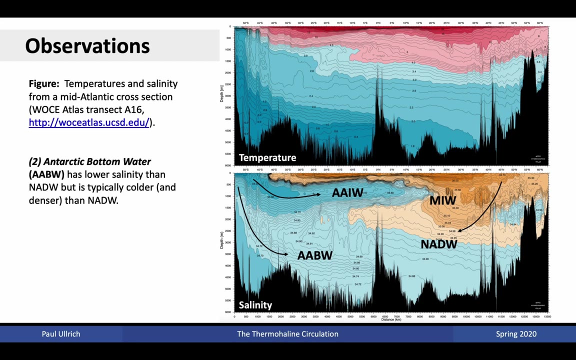 Antarctic Circumpolar Current. However, because they are not also associated with brine rejection and other deep polar processes, these waters are typically more buoyant than water at depth. The second type of water is the Antarctic Bottom Water, or AABW. This is typically lower. 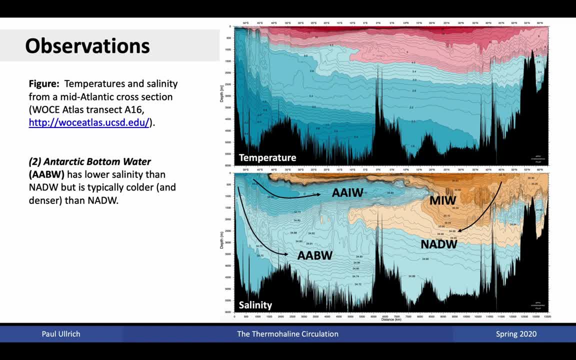 salinity than the North Atlantic Deep Water, but is typically colder and denser than NADW as well. Antarctic Bottom Water primarily forms in the deep polar, which is the polar regions of the South Atlantic, such as the Wendell Sea, Along the interface of, for instance, sea ice. we have processes that are then responsible for. 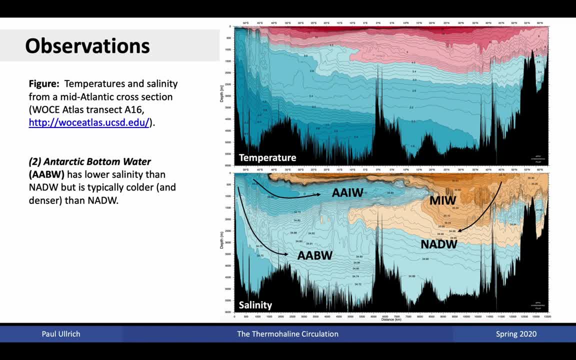 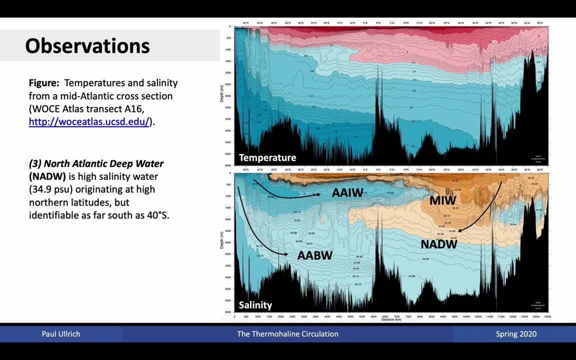 driving up density and consequently driving water to depth. The third type of water is the North Atlantic Deep Water, or the NADW. This is typically very high salinity water that originates at high northern latitudes. Typically, this is responsible for the highest salinity water in the Arctic. This is typically the highest salinity water. 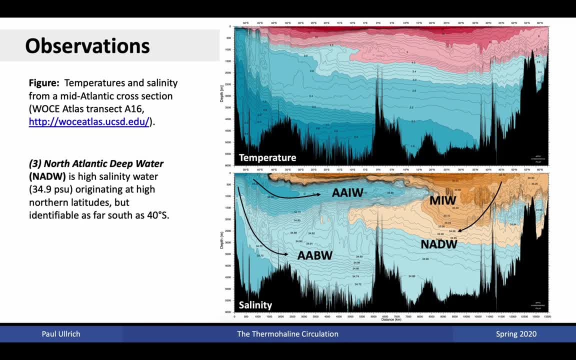 at depth and it's identifiable as far south as 40 degrees south. In the diagram on the right, the region of North Atlantic Deep Water corresponds roughly to the brown contours. North Atlantic Deep Water is very saline, again through brine rejection processes. 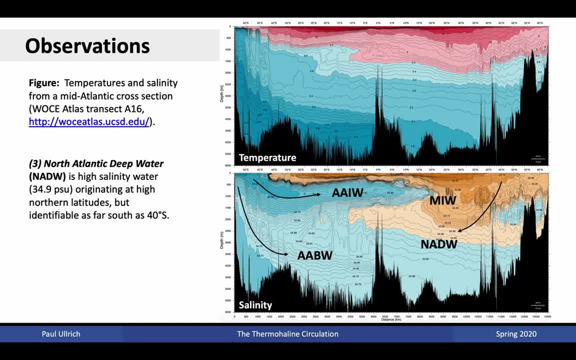 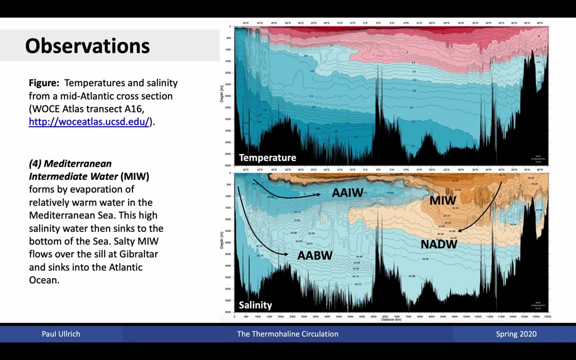 and simply because the North Atlantic tends to be very saline. North Atlantic Deep Water primarily originates from the Labrador Sea and the Greenland Sea. The last water that we see in this diagram is the Mediterranean Intermediate Water, or the MIW. This forms because of evaporation of the relatively 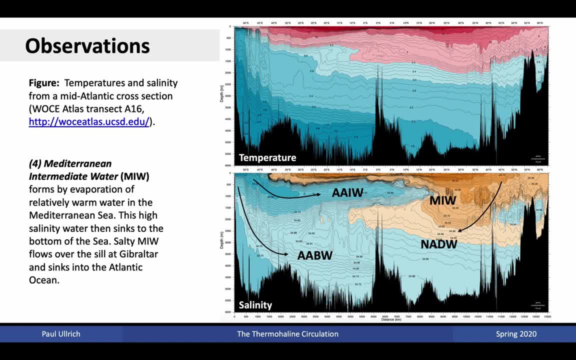 warm waters in the Mediterranean Sea. Recall from before that the Mediterranean Sea is abnormally saline compared to some of the other inland seas, as well as being relatively saline compared to the similar vicinity in the North Atlantic. The high salinity water from the Mediterranean 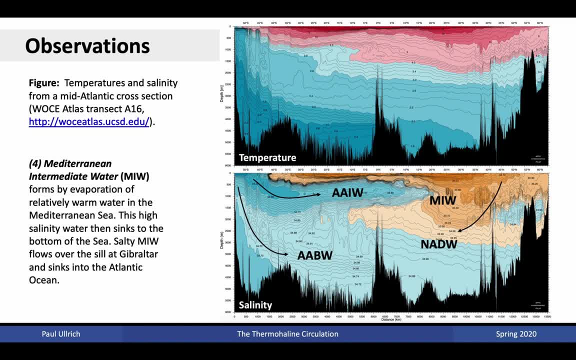 sinks to the bottom of the sea and it then passes over the sill at Gibraltar and sinks in the Atlantic Ocean. This water can reach as far west as Bermuda. The four different Atlantic Ocean waters can also be seen in the dissolved oxygen content in the. 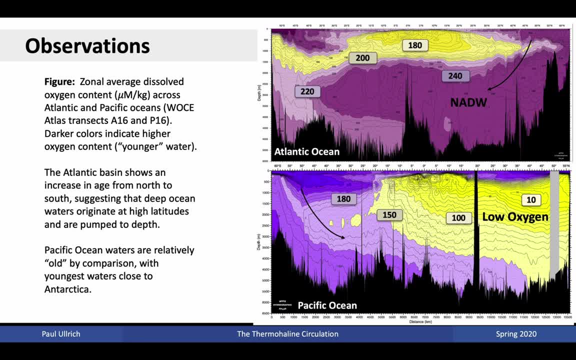 Atlantic. Here on the top diagram we see that dissolved oxygen content in micromoles per kilogram in the Atlantic and on the bottom in the Pacific. What we see is that regions that were more recently exposed to the surface tend to have a higher oxygen content associated with them. 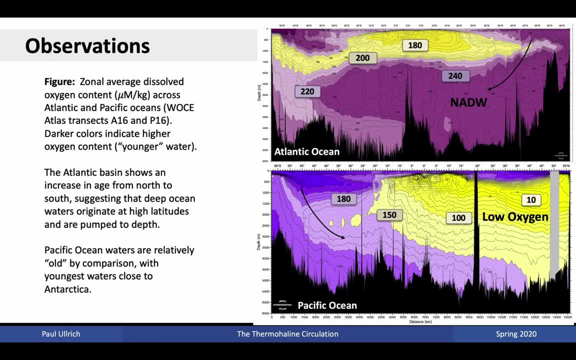 In particular, this in North Atlantic deep water has some of the highest oxygen content of the Atlantic Ocean waters. at depth, The Atlantic basin generally shows an increase in the age of water from north to south, suggesting that these deep ocean waters typically originate at high latitudes. 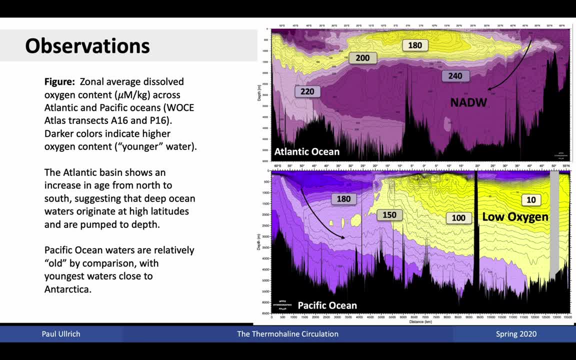 in the northern hemisphere and are pumped to depth In the Pacific. on the other hand, we see a very different picture. Namely, we see incredibly low oxygen content in the Pacific at depth in the northern subpolar latitudes. In fact, we see the highest oxygen contents occurring in the south of. 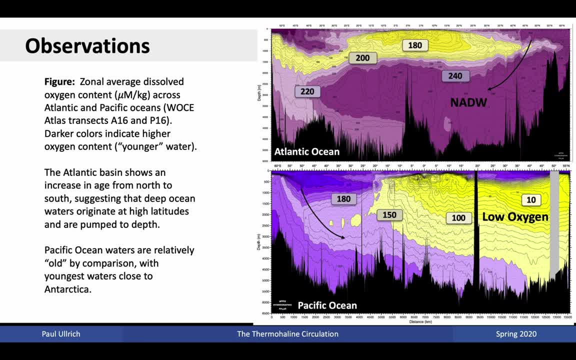 the Pacific Ocean near the Antarctic Circumpolar Current. This is indicative of relatively older waters through the Pacific and also seems to indicate that most of the Pacific deep water exchange comes from the south and moves to the north, with oxygen basically being depleted over the course of its movement. Consequently, we see that at depth, then at North Atlantic waters. 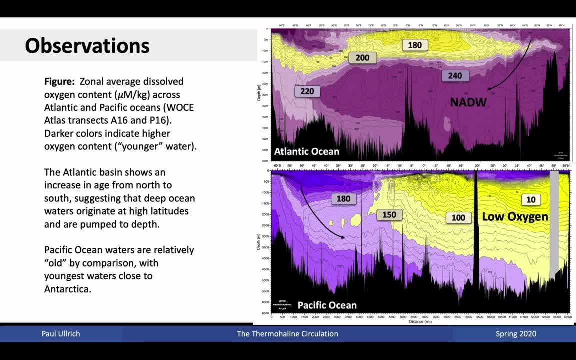 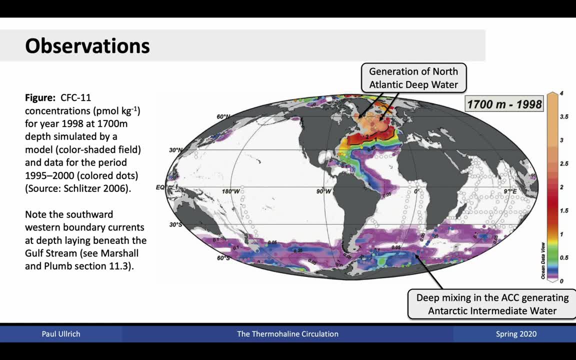 tend to move south, whereas in the Pacific, the south-pacific moderate waters are those that typically move north through this basin. Finally, looking at chlorofluorocarbon concentrations in picomole per kilogram, we see evidence of the highest CFC concentrations occurring in the North. 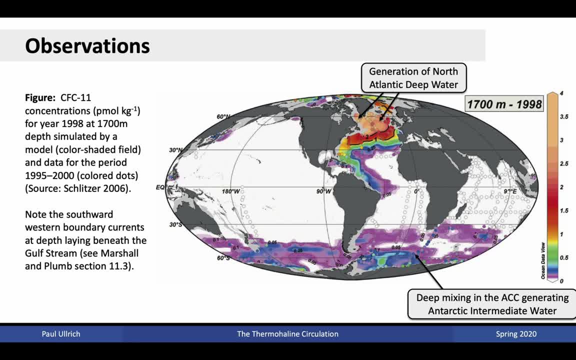 Atlantic and some evidence of CFCs also in the South Atlantic. along the Atlantic, the Antarctic circumpolar current Generation of North Atlantic deep water in the Labrador Sea and Greenland Sea are primarily responsible for pumping air containing chlorofluorocarbons. 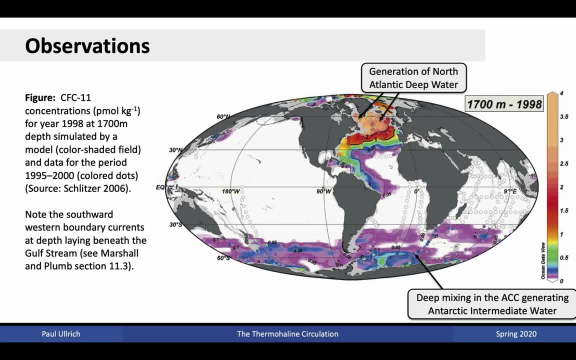 to depth, hence resulting in this gradient of concentrations. The highest concentrations of CFCs occur roughly in these regions, where we have the deepest mixed layers, and thus those regions that are associated with the deep convection. From there, we see the CFCs spread out at depth. 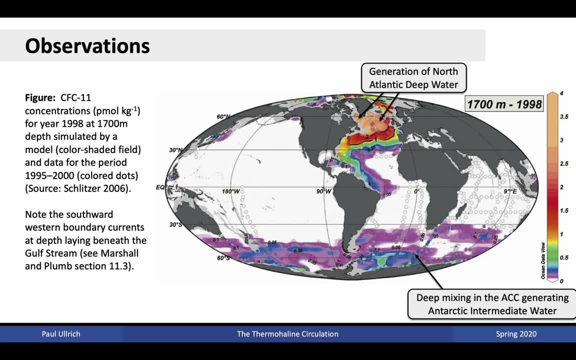 with CFC concentration roughly increasing as we move from the North Atlantic to the South Atlantic. The pattern of CFC concentration is also indicative of the deep ocean currents that arise in the Atlantic. Recall that we have a strong western boundary current in the near surface Atlantic, known as the Gulf Stream. This is responsible for pumping warm ocean waters from. 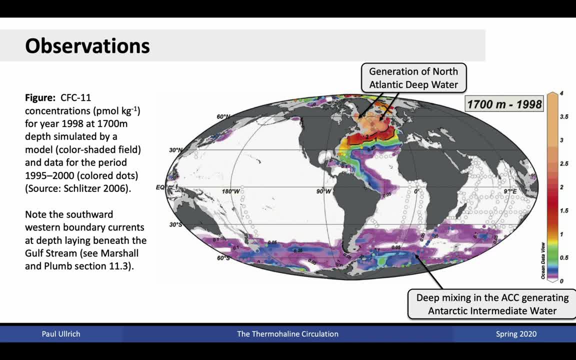 the south into the polar regions, Correspondingly at depth. we also have a deep concentration of CFCs. The CFC concentration is also indicative of the deep ocean currents, that current that underlays the Gulf Stream, This deep western boundary current is instead responsible. 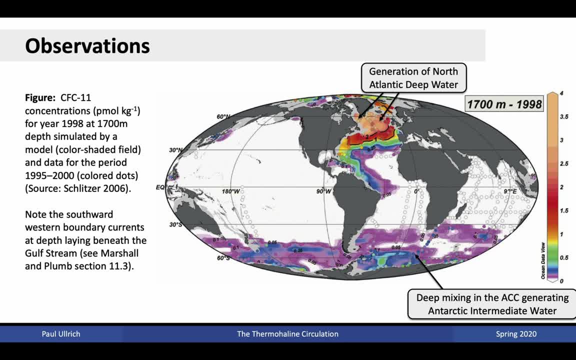 for pumping oceanic waters from the subpolar regions southwards along the western boundary. We can see clear evidence of it here, as it's responsible for transporting these CFCs from the North Atlantic waters southwards In the southern hemisphere. the CFC concentrations 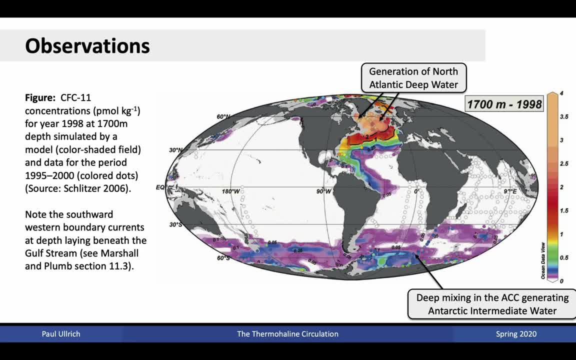 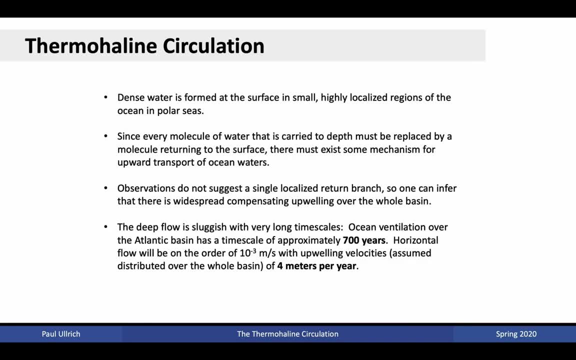 at depth are primarily driven by particularly deep mixed layers that occur along the Antarctic circumpolar current. All right, so let's review. The thermohaline circulation is associated with dense water that is formed at the surface in small, highly localized regions of the ocean, in the polar. 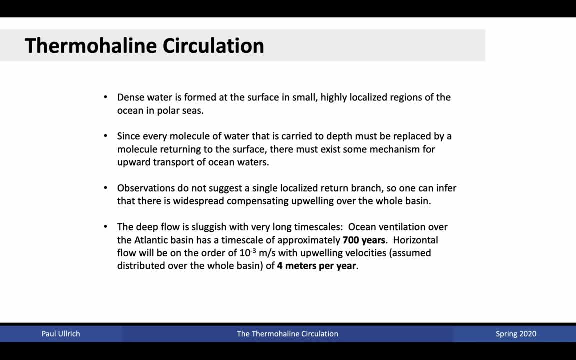 seas, specifically in the Labrador Sea, the Greenland Sea and the Wendell Sea in the South Atlantic, Since every molecule of water that is carried to depth must be replaced by a molecule returning to the surface, that is, since we have conservation of oceanic. 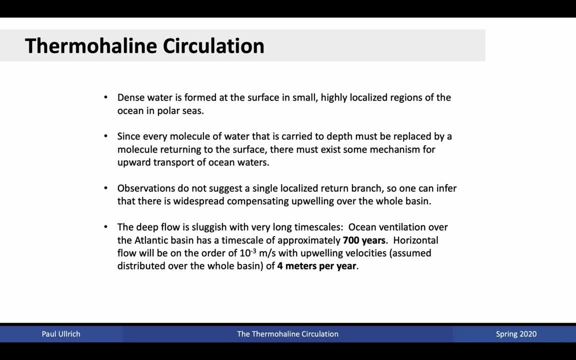 water mass. there must exist some mechanism for the upward transport of ocean waters. Since observations do not suggest a single localized return branch, that is, we do not have a upwelling or convective action which is responsible for bringing deep ocean waters back to the surface, we must infer that there is instead widespread compensating upwelling. 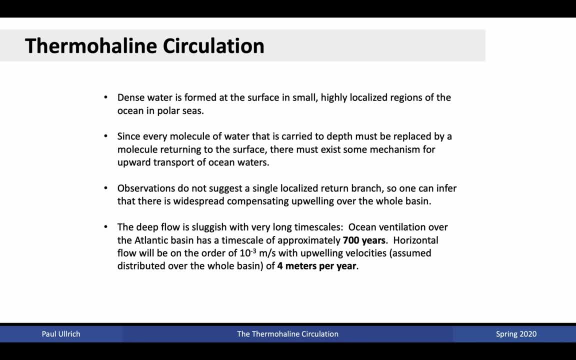 that occurs over the whole basin, That is, away from these regions of deep convection, the ocean waters are slowly able to return to the surface. This deep flow is sluggish and with very long timescales associated with it. Ocean ventilation of the whole Atlantic basin has a timescale of approximately 700 years, That is, if we were to. 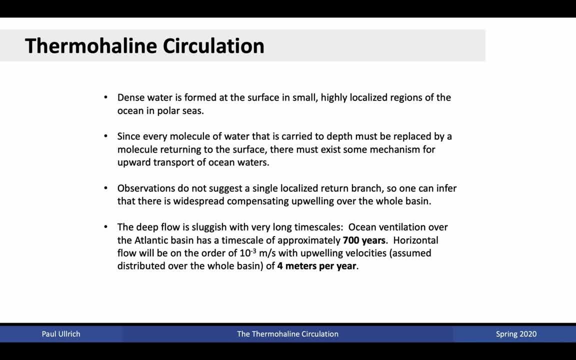 look at chlorofluorocarbon concentrations 700 years from now, we would see finally approximately uniform distributions of that chlorofluorocarbon density. The horizontal flow is on the order of about 10 to the minus 3 meters per second, or millimeters per second with upwelling. 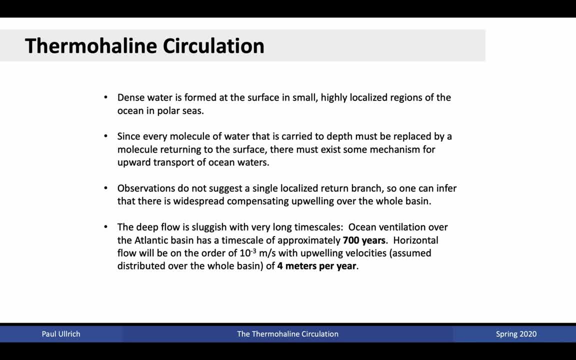 velocities, distributed over the whole basin, of approximately 4 meters per year. These upwelling velocities obviously cannot be observed directly and are instead inferred simply from conservation of mass. The general picture that we get of the thermohaline circulation again appears here. 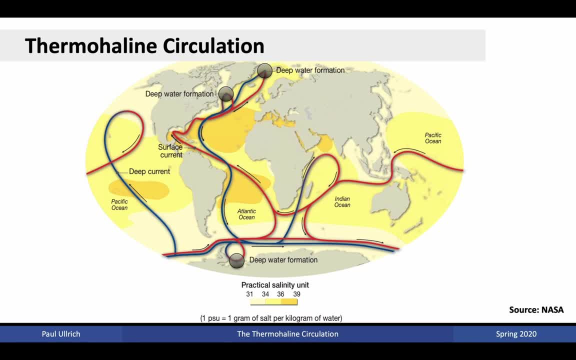 This is again an idealization. There are a few things to take home from this, though, In particular, localized regions of deep water formation as depicted on the map, strong western boundary currents, particularly the Gulf Sea stream, that occur in the Atlantic, and returning branches of those western boundary currents. 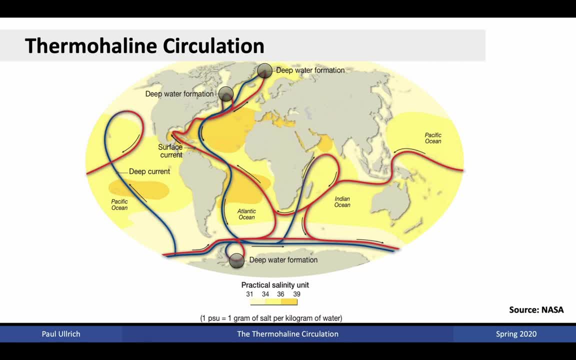 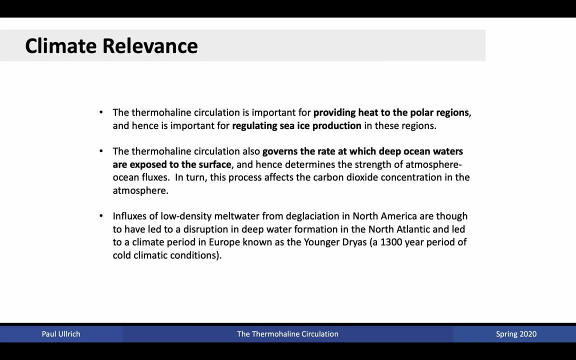 underlaying them at depth. This is primarily responsible, then, for circulating ocean waters. through the Atlantic As well. we see large-scale upwelling of oceanic waters at depth back to the surface. that occurs in effectively all of the ocean basins, So the thermohaline circulation. 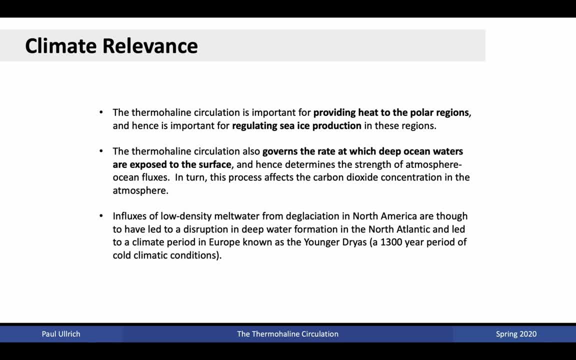 is important on a climatological scale because it provides heat to the polar regions. That is, the thermohaline circulation provides a mechanism for ocean waters to leave the polar regions at depth. Without the thermohaline circulation, the Gulf Stream would likely. 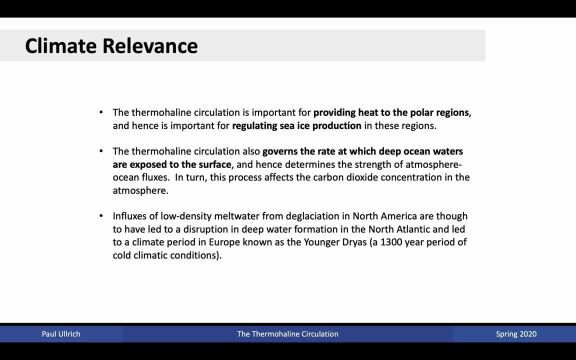 be significantly weakened. Hence the thermohaline is important for regulating sea ice production, because it is responsible for bringing warmer ocean waters into the polar regions, where that heating can then reduce sea ice production. If one assumes that the thermohaline did not exist, 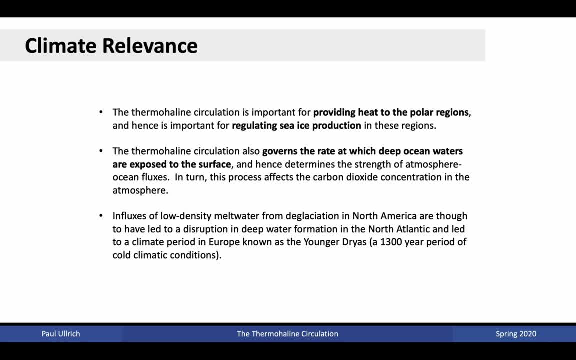 then we would have to think about the possibility of the thermohaline circulating in the Arctic. It would have much weaker surface currents for bringing those warm waters northwards. A shutdown of the thermohaline circulation would then lead to much colder ocean waters through. 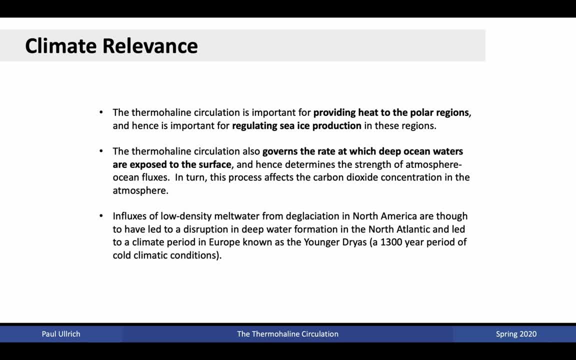 the Atlantic Ocean, and hence a more southern extent of sea ice production. The thermohaline circulation also governs the rate at which deep ocean waters are exposed to the surface. Hence it provides a mechanism in order to bring tracers from the surface to depth. 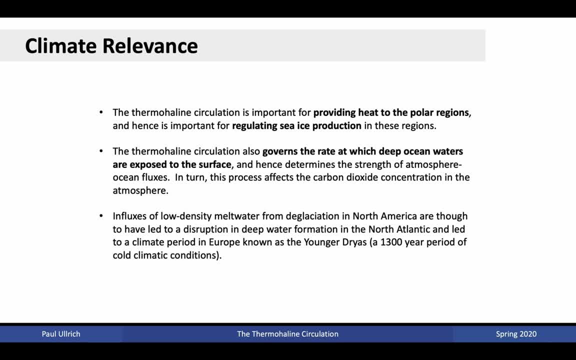 as well as a mechanism to bring energy from the surface to depth. Consequently, surface warming that may occur under climate change can translate to warming at depth over a very long timescale, process by which the deep convection effectively transports this energy to depth where it can be stored in the ocean. 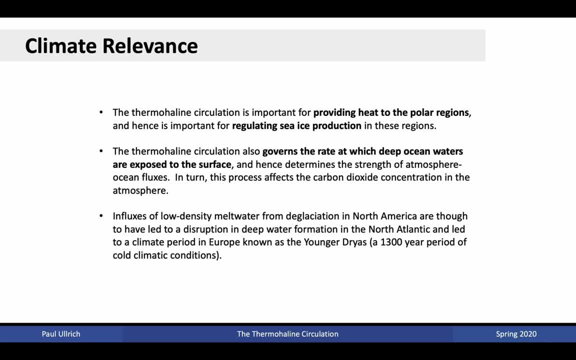 The thermohaline circulation also determines the strength of these atmosphere-ocean fluxes, because of this governing the rate at which surface and deep water is extremely rich. In turn, this process also affects carbon dioxide concentrations in the atmosphere, because the ocean acts as a buffer or storage mechanism for carbon dioxide. 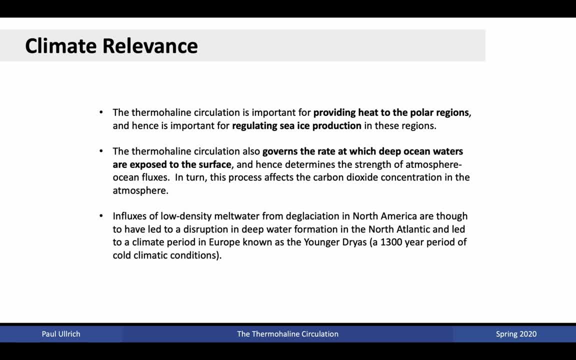 Influxes of low-density meltwater from deglaciation of North America that occurred at the end of the last glacial phase were known to disrupt the formation of deep water in the North Atlantic by injecting fresh water and hence blocking the process that leads to the formation of relatively 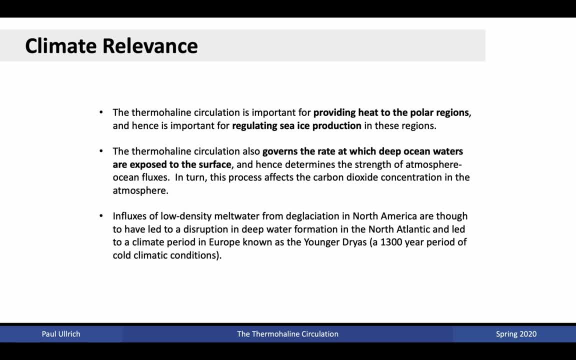 dense surface waters. This process is known to disrupt the formation of deep water in the North Atlantic by injecting fresh water and hence blocking the process that leads to the formation of relatively dense surface waters. This then led to a period known as the Younger Dryas, which was a 1300 year period of abnormally 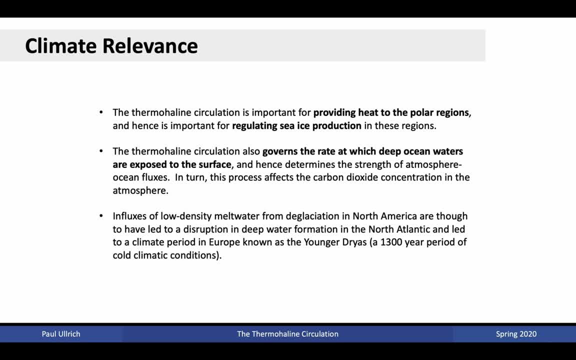 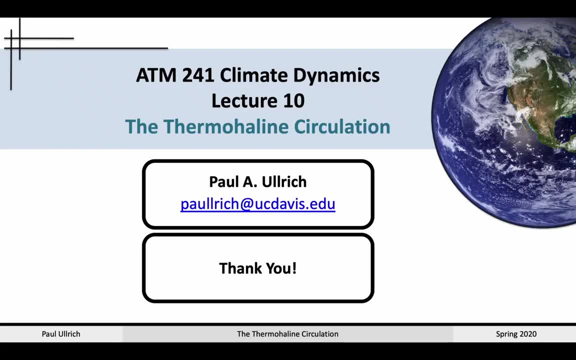 cold climatic conditions. The primary driver for this period was then thought to be an effective shutdown of the thermohaline circulation. Alright, that's everything for today. That concludes our discussion of the ocean topics in this class. Next time we'll be talking about 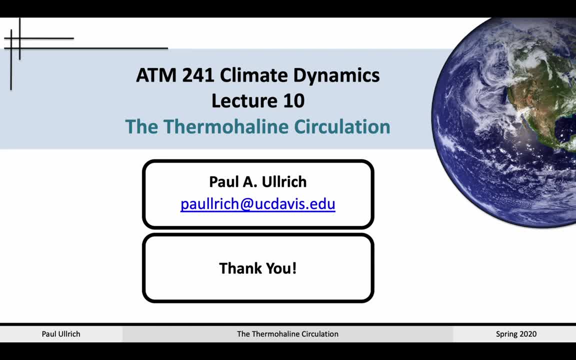 climate dynamics, bringing together atmosphere-ocean interactions in order to better understand the climate system. Thank you.